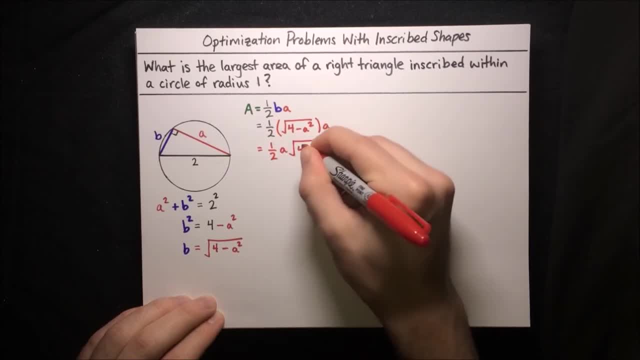 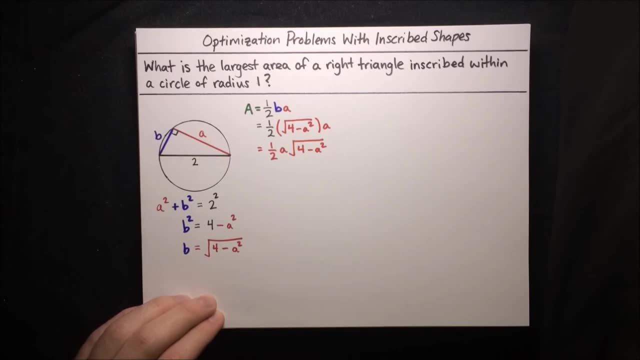 one half times a times square root of four minus a squared. Okay, so now we've got an expression for the area of the circle in terms of a single variable, And now we can maximize it by finding its stationary points. So we'll take the derivative. 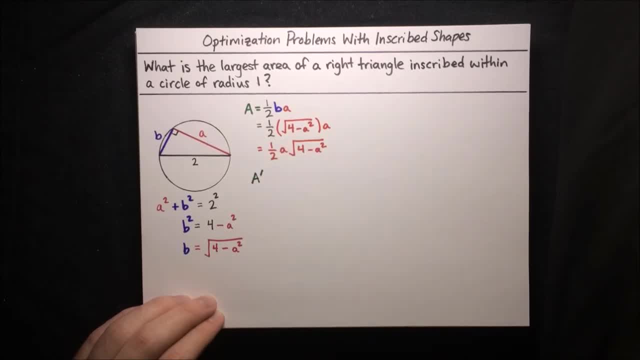 a prime that's just going to come from the product rule. So it'll be equal to the derivative of the first term, A half, a derivative of that times root of four minus a squared, And then plus the first term, a half a times the 되�. 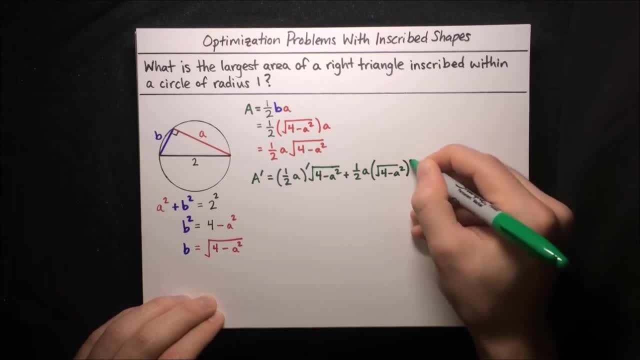 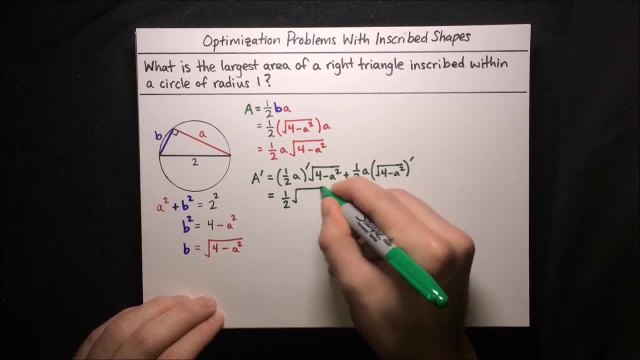 derivative of 4 minus a squared And we'll go ahead and do that computation. So derivative of 1 half a is just a half. So 1 half square root of 4 minus a squared and then plus 1 half a. 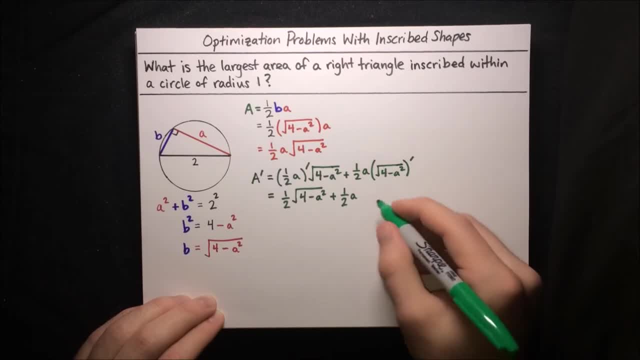 and then derivative of this thing. So the root is really like a half power. So that'll come out 1 half, and then we'll have that 4 minus a squared to the power of a half minus 1, which is negative half, And then we've got a chain rule it. so multiply by the derivative. 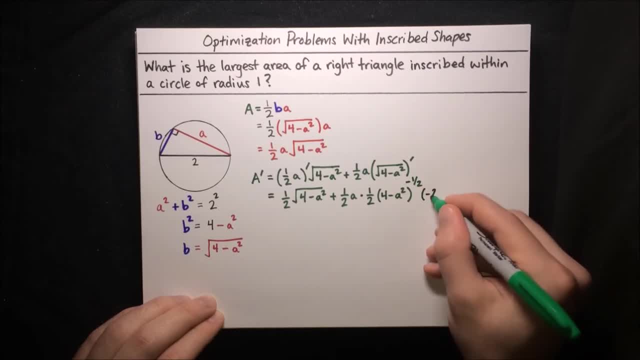 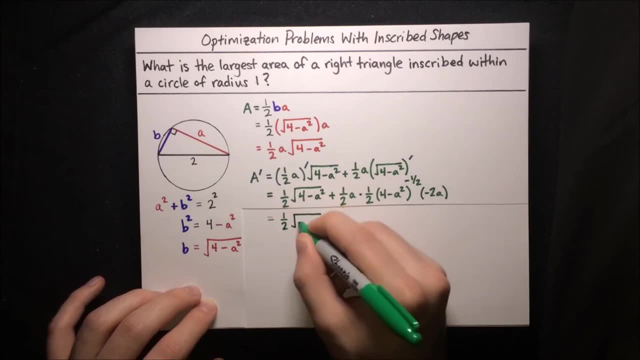 of the inside, which is negative 2a. So we simplify and then we find that this is equal to a half square root of 4 minus a squared, minus a squared over 2 times the square root of 4 minus a squared. And we want to find the stationary points, which means we want to 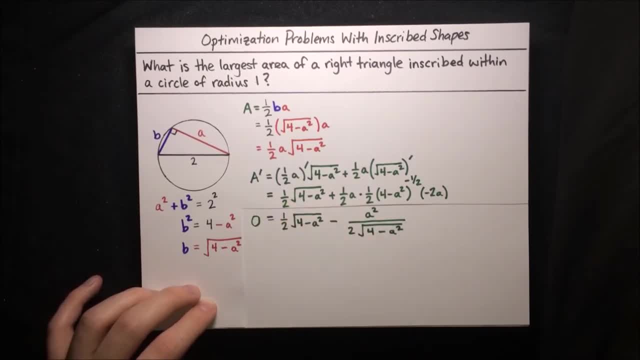 set that derivative of 4 minus a squared to the power of a half square root of 4 minus a squared. Now, as is, this equation looks a little rough because of all of these square roots, But something that we can do to simplify this all is to multiply by this square root of 4. 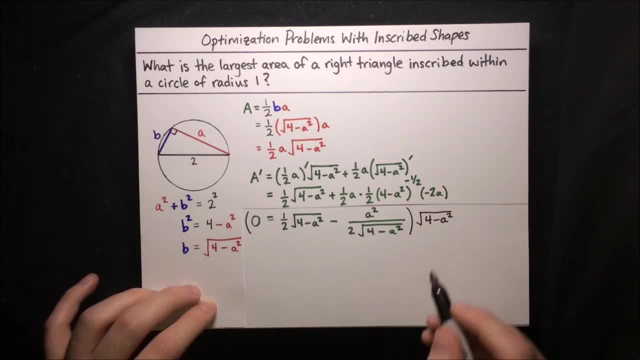 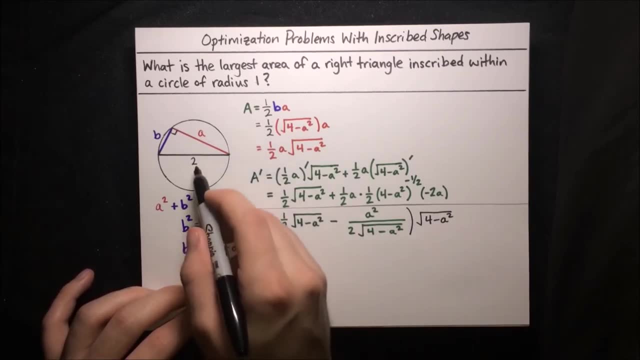 minus a squared, And we are allowed to do that because we know that this is not 0.. a squared is not equal to 4 because a is not equal to 2, because 2 is the hypotenuse of this triangle, whereas a is just a leg, And the leg is always smaller than the hypotenuse. 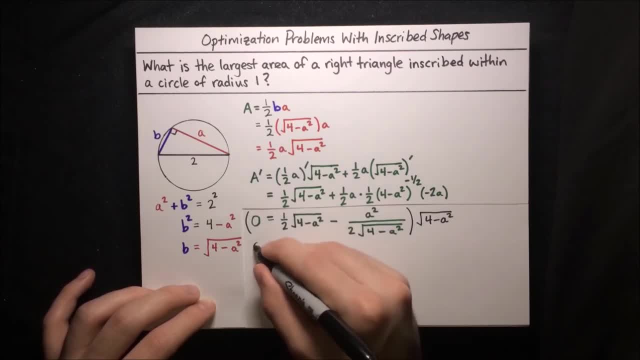 So we go ahead and multiply by the derivative of 4 minus a squared And we find that this is equal to a half square root of 2 minus a squared. by root four minus a squared. That simplifies the equation a lot. We just have 0 equals 1, half times for minus a squared and then minus a squared. 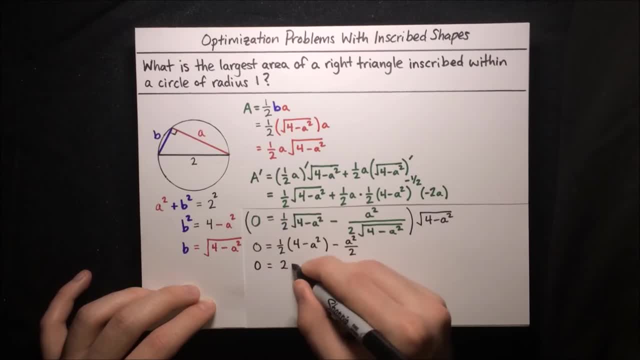 over two, which is a lot easier to solve with. 0 equals two minus one half a squared, minus our a squared over tw. Let's write that as 1 half a squared and negative 1 half a squared, negative half a squared. those combine into just minus a squared. 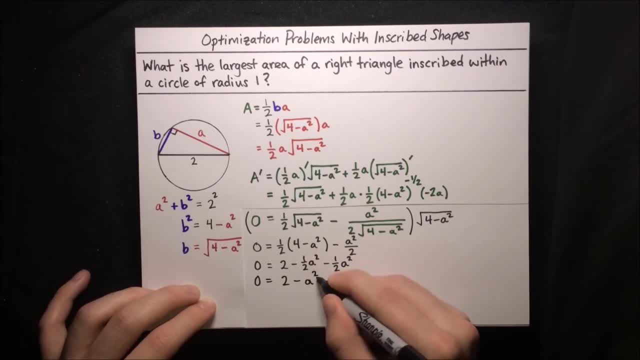 0 equals 2 minus a squared, which means a squared equals 2,, which means a equals the square root of 2, the positive root, since a is a physical length. here You can check that this value is indeed a maximum of our area function by using the first or second derivative test, and I assure you it. 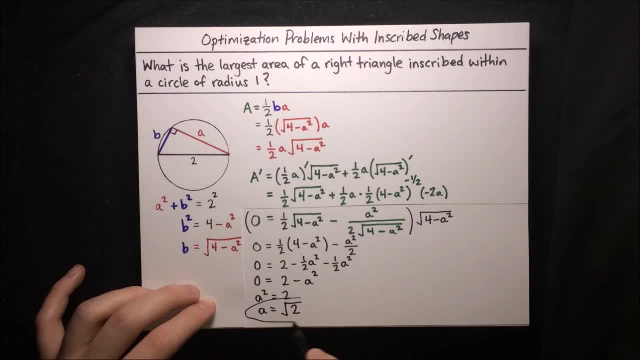 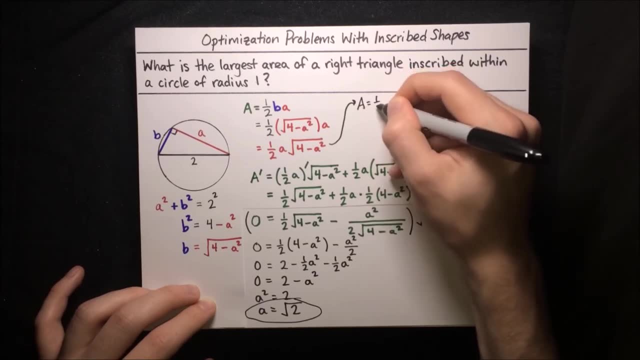 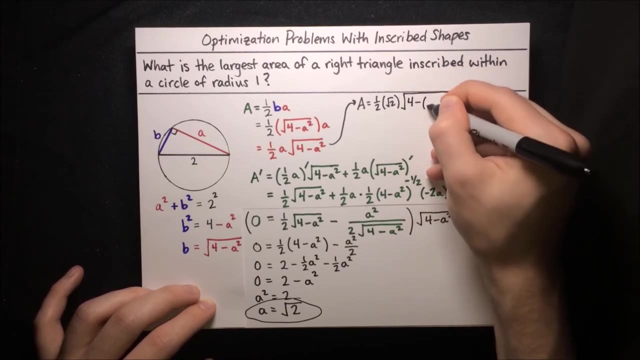 will work out. So now we're pretty much there. we just have to plug this value back into our area function here and that will give us the largest area. So area equals one half times a, which is root 2, times root of 4 minus a squared a again is just root 2, and we're scoring that. so this 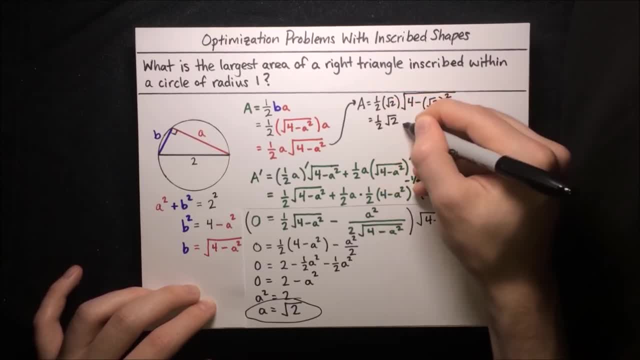 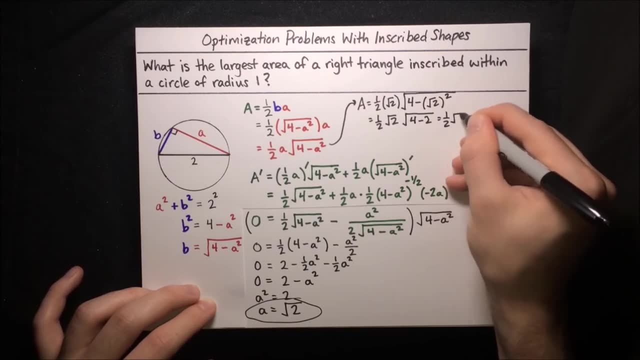 becomes one half times root 2, times the root of 4 minus root 2 squared, which is 4 minus 2, which is equal to one half root 2 times root 2, which is equal to one half squared Times two, which is equal to one. So there we go. that is the largest area of a right. 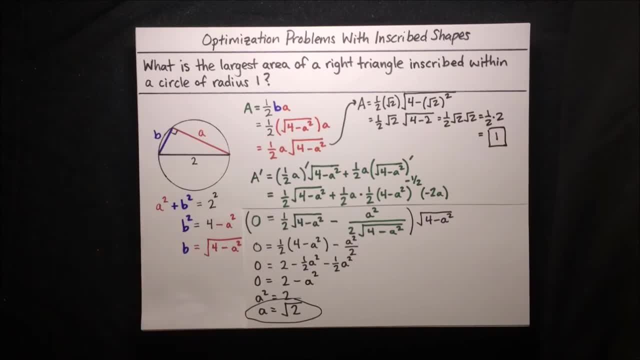 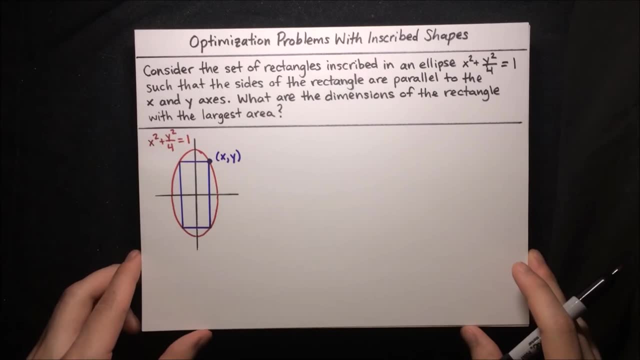 triangle inscribed within a circle of radius one, The area is equal to one. Here's our next problem. We want to consider the set of rectangles inscribed in an ellipse. x squared plus y squared over four is equal to one, such that the sides of the rectangle are: 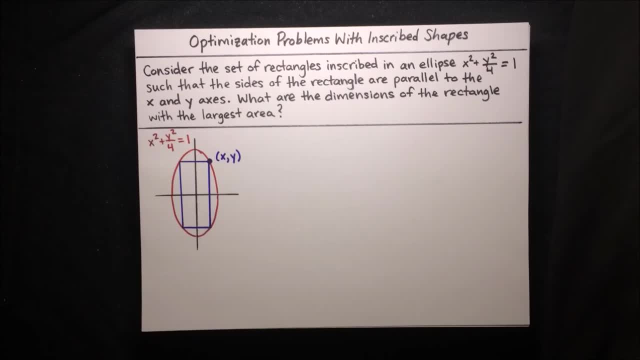 parallel to the x and y axes, And we want to know what are the dimensions of the rectangle with the largest area. So here we've got a diagram of our ellipse and a rectangle inscribed within it, and why don't we say the corner point of the rectangle in the first quadrant is xy? The first thing that we want to do 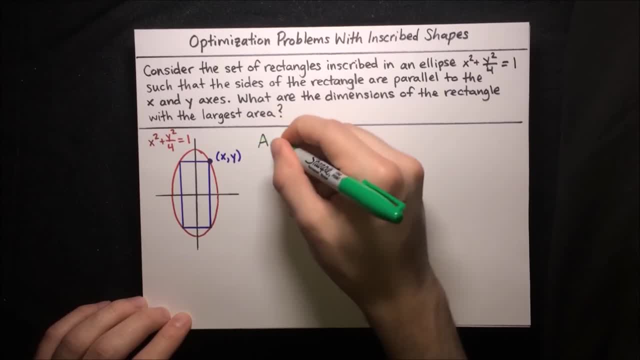 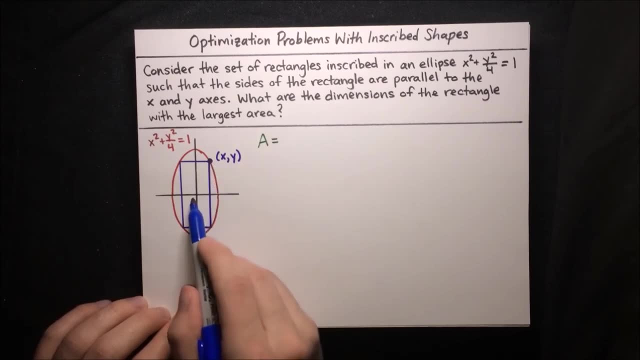 is to write our area function, because that's what we want to maximize. So area equals what? Well, area equals base times height for this rectangle. and if we know the distance from the origin to the right side of the rectangle is x, then the base consists of two of those distances. 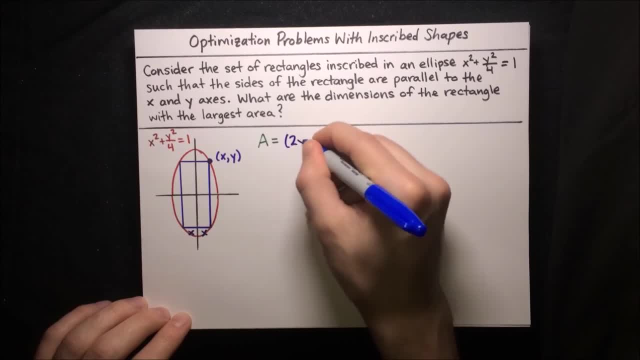 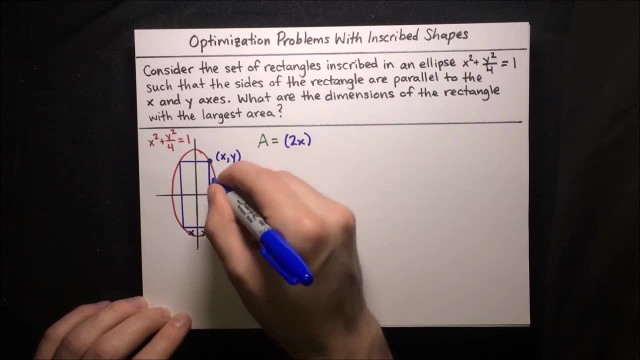 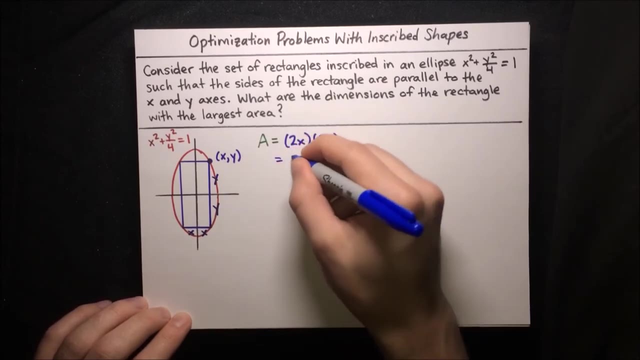 x and x. so base is 2x and then height. if we know, the distance from this x axis up to the top side of the rectangle is y, then this is y, and so is that y and y. we've also got 2y, So that means area is equal to 4xy. 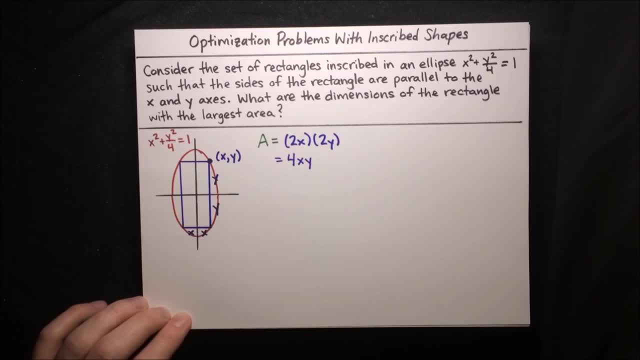 And, of course, we want to express this area function in terms of a single variable, because we want to maximize it. Thankfully, we have an equation that we can use to solve for x or y in terms of the other. We've got x squared plus y squared over 4y, and we've got x squared plus y squared over 4y. 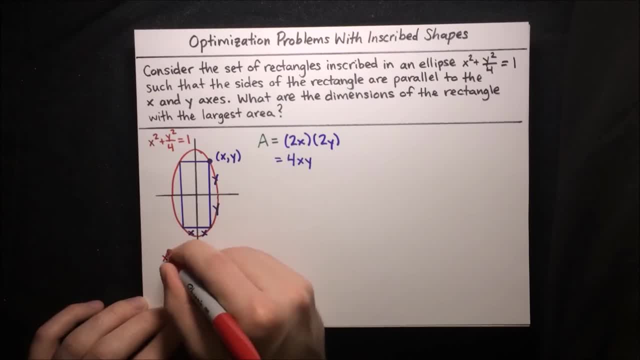 equals 1.. So why don't we start with that equation: x squared plus y squared over 4 equals 1.. Let's clean it up a bit: multiply by 4 to get rid of the fraction, So 4x squared plus y squared. 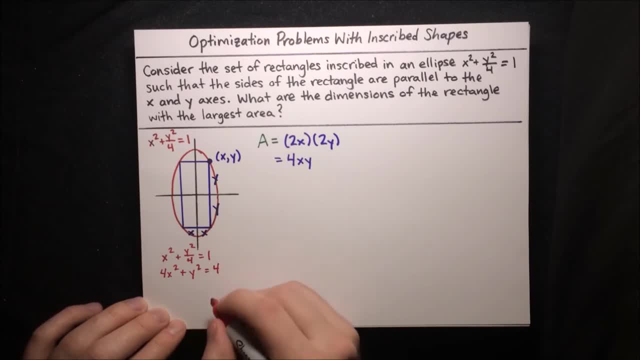 is equal to 4, and why don't we just solve for y squared, So y squared is equal to 4 minus 4x squared. Solve for y: y equals the square root of 4 minus 4y, 4x squared, a positive root, since we want it to represent a length, So we plug this in. 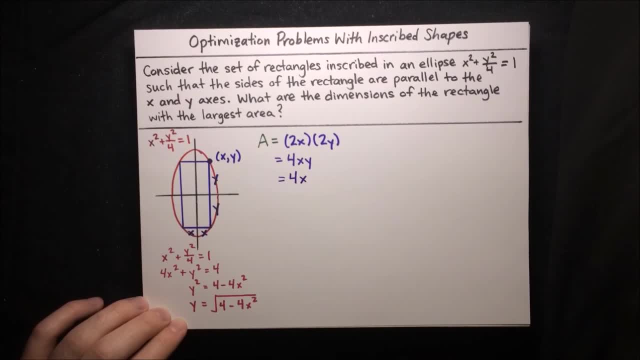 we find that the area is equal to 4x times y and y is just the root of 4 minus 4x squared. So now we've got our area function in terms of a single variable and we can differentiate using the product rule. So derivative of area is equal to the first term, differentiated 4x derivative. 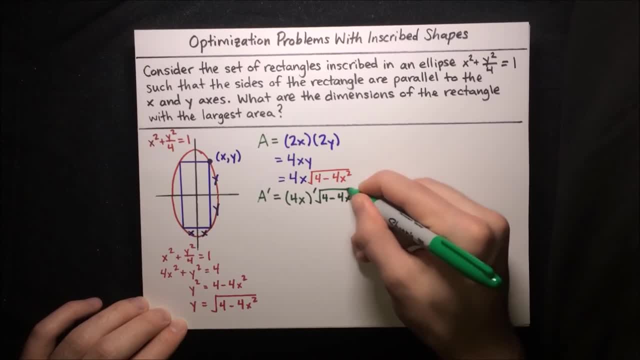 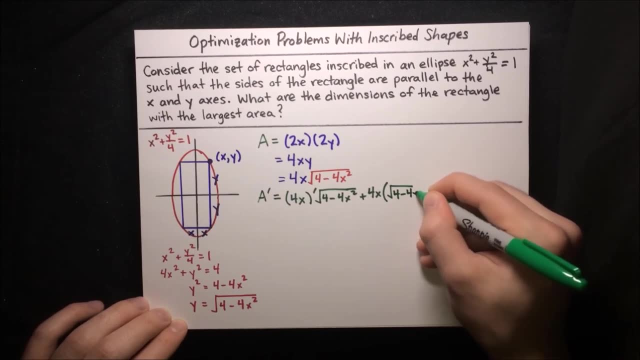 squared of 4 minus 4y, 4x squared and then plus 4x times that second term differentiated. So square root of 4 minus 4x squared derivative. Now this first term, that's easy derivative of 4x is just 4.. So 4. 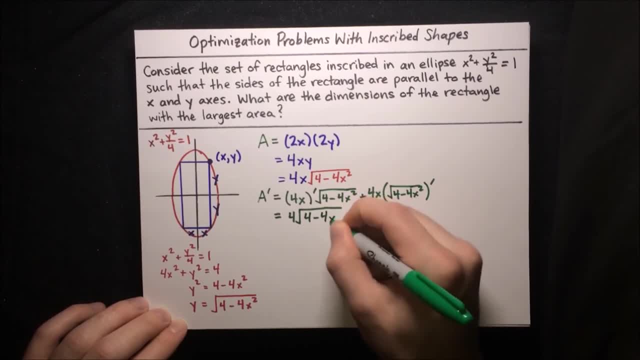 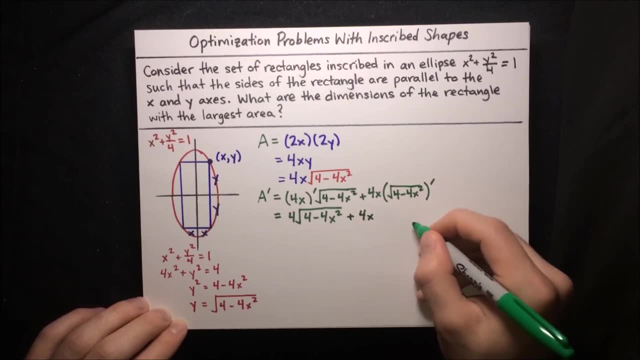 root: 4 minus 4x squared, and then the second term is a bit tougher, but it's still doable. The root is like a power to the one half. so bring that down: part of the power, rule one half. 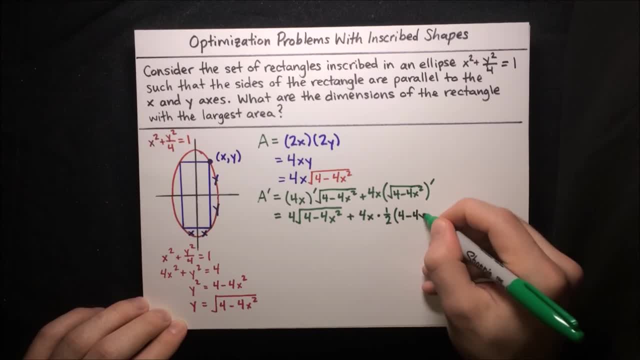 times that original expression inside the root, 4 minus 4x squared, and then decrease that exponent of a half by one, you get negative one half. and then you've got to apply the chain rule to the inside, the derivative of the inside of the root, the derivative of 4 minus 4x squared. 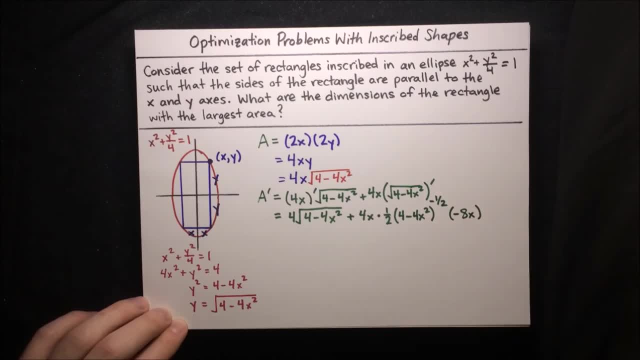 is just negative 8x using the power rule. So we go ahead and simplify all of that. we get 4 root of 4 minus 4x squared, and then minus 6x squared, 16x squared over the root of 4 minus 4x squared. So there we go. that is the derivative, and to 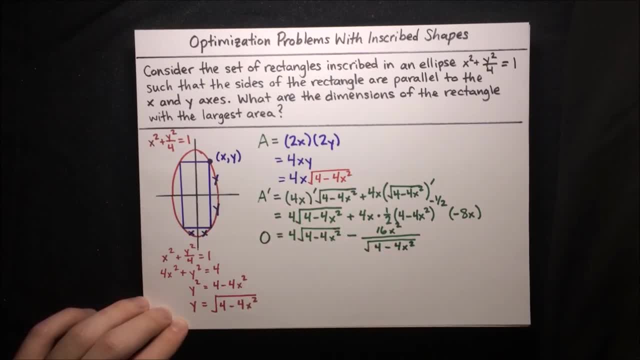 find the stationary points. we want to set that derivative equal to 0 and solve. And again we will go ahead and multiply by this square root to clean up the equation a bit. multiply by square root of 4 minus 4x squared. We know we're allowed to do that because it's non-zero, and we know that. 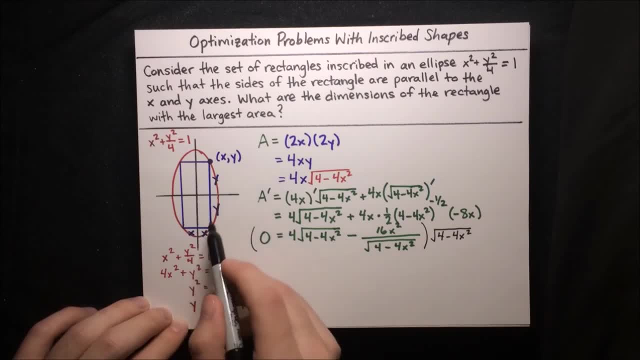 because x can never be equal to 0. So we're allowed to do that because x can never be equal to 0. Otherwise, if x were 1, the x would lie perfectly on the x-axis and we would just have a line. 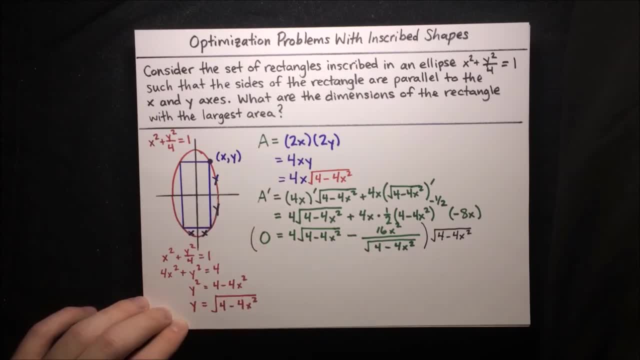 segment across. So that's definitely not the case. So we go ahead and simplify this equation. we get that 0 equals 4 times 4 minus 4x squared. the roots cancel and then minus 16x squared because the denominator cancels. So we go ahead and solve this: 0 equals 16 minus 16x squared. 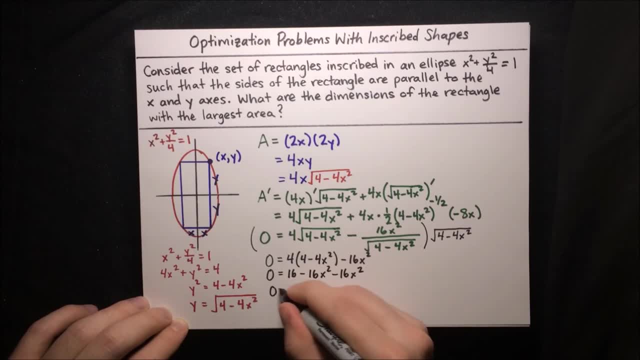 so 0 equals 16 minus 32x squared. Let's bring that up here to continue solving. So 32x squared equals 16, that means x squared is equal to 1 half, which means that x is equal to the square. 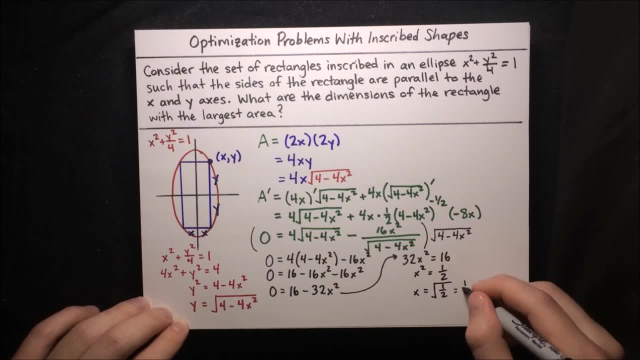 root of one half, which simplifies to 1, over square root of two, which simplifies to square root of one half. So we get equal to 2s. squared we Greater than equal to 1 minus square root of 2,. 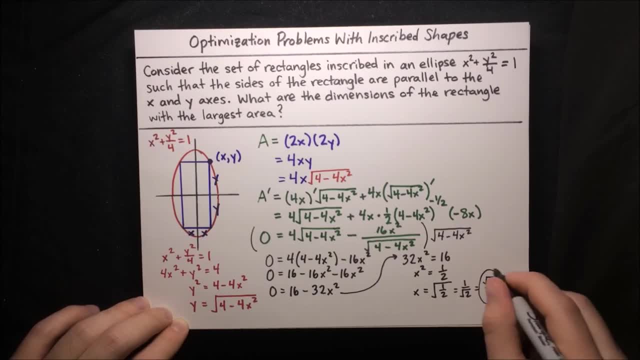 of 2 over 2.. So that's our value for x, and you can check that this is a maximum of the area function by using the first or second derivative test. I assure you it will work out. Now all that remains is to figure out what is y, and to do that, all we need to do